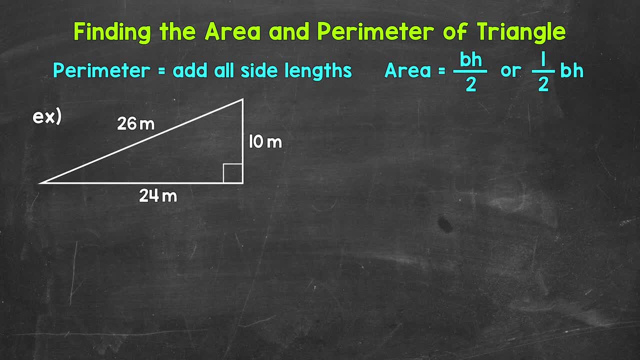 area of a triangle. we use the formula base times height divided by 2, or 1 half times base times height. Dividing by 2 and multiplying by 1 half give us the same result, so either formula works and will give us the correct area. I'm going to use base times height divided by 2. 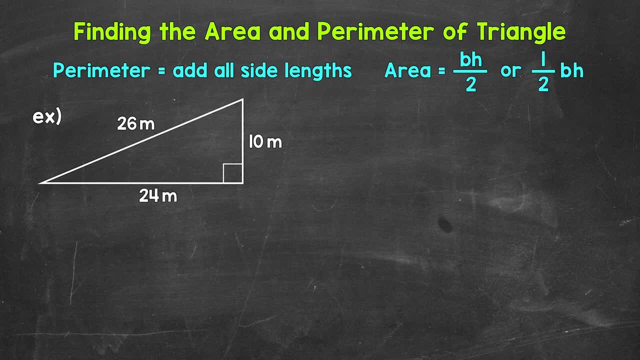 in this video. Now I do go into more detail about finding the area of triangles and the area of the triangle. but I'm going to go into more detail about finding the area of triangles and the area of the triangle. this formula in another video. that link is in the description for this video. i'll go through two. 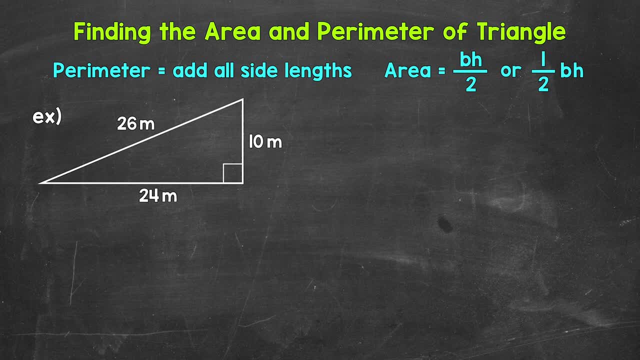 examples. let's jump into number one, where we have a right triangle and we will start with perimeter. again, we need to add all of the side lengths in order to find the perimeter. so a triangle has three sides, so we need to add all three of those side lengths, so perimeter equals well, 24 meters. 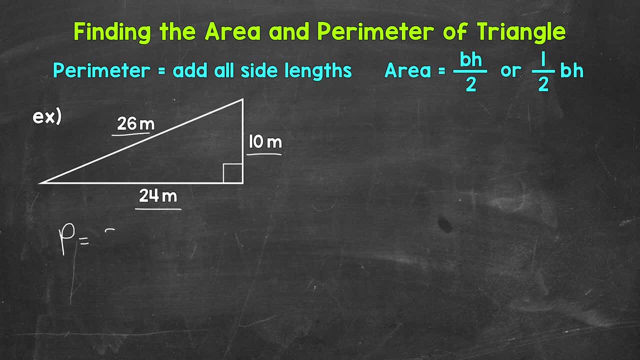 plus 26 meters plus 10 meters, so 24 plus 26 plus 10. now it doesn't matter what order you add the sides in, so something to keep in mind, you'll get the correct perimeter however you do it. so 24 plus 26 gives us 50 plus 10 gives us a perimeter of 60 meters. 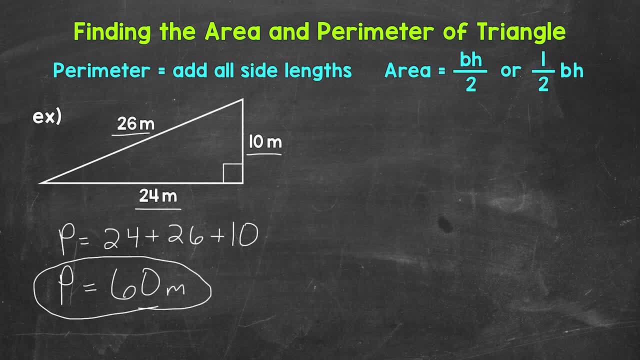 we will start with the formula, so area equals base times height divided by 2.. let's move on to finding the area of this triangle. we will start with the formula, so area equals base times height divided by 2. we're going to use 24 for the base and 10 for the height. we do. 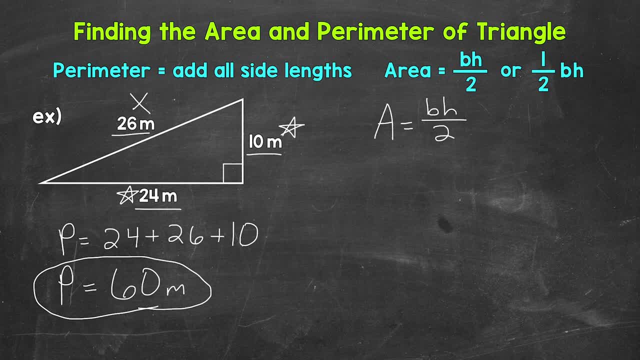 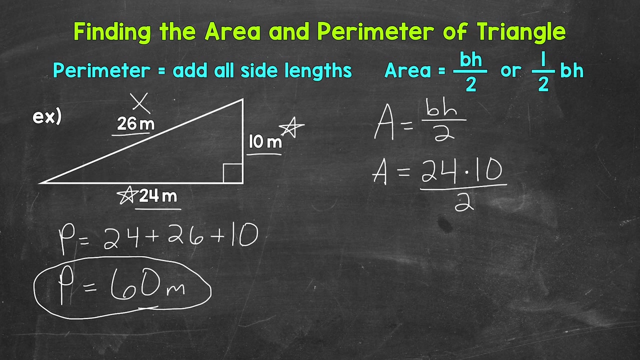 not need this 26 meters in order to calculate the area. Again, 24 meters for the base and 10 meters for the height meters for the corresponding height. so let's plug in 24 for the base, times 10 for the height divided by 2.. so now we can work through this. let's do 24 times 10 next, which gives us 240. 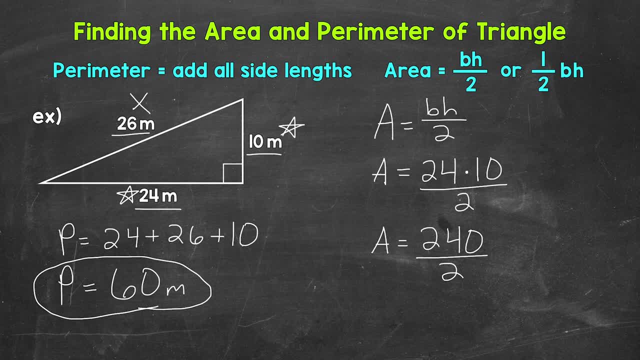 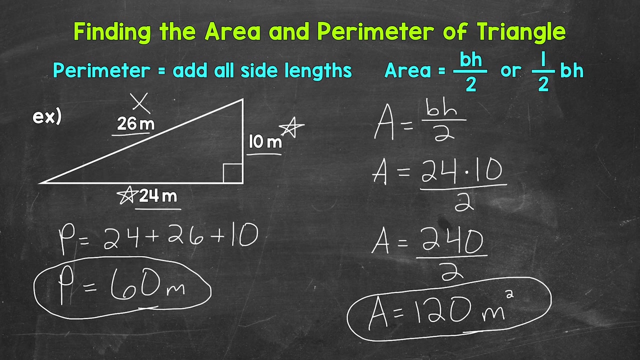 so we have 240 divided by 2, that gives us an area of 120 square meters. so for this triangle we have a perimeter of 60 meters and an area of 120 square meters. let's move on to another example. here is our second example. let's start by 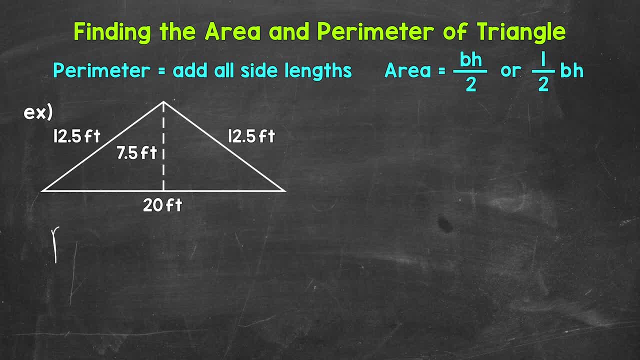 finding the perimeter, so perimeter equals. and then we need to add all of the side lengths, so we have twelve and five tenths, or twelve and a half feet right here, twelve and five tenths, or 12 and a half feet right here, and then 20. 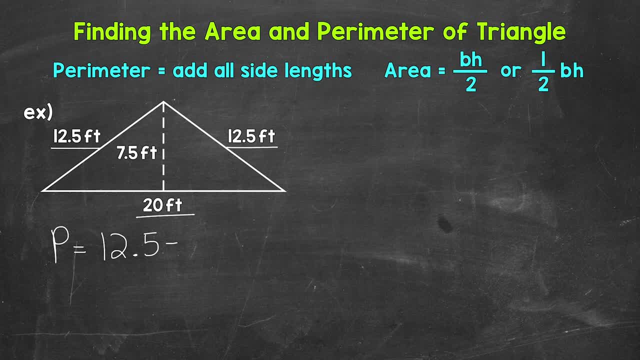 feet. so let's add all of these side lengths. now, keep in mind we do not need this seven and five tenths feet or seven and a half feet right here. That's the height that we will use for the area. That's not one of the side lengths, So we do not need it for perimeter. 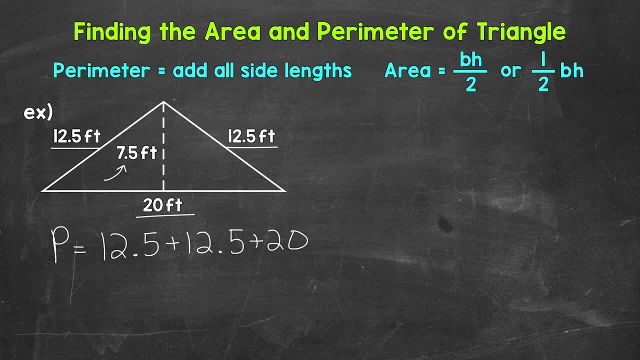 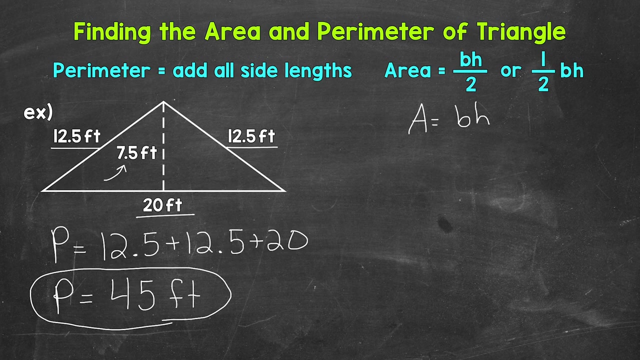 Now let's add all of these side lengths. So twelve and a half plus twelve and a half gives us twenty. five plus twenty gives us a perimeter of forty five feet. Let's move on to area. So area equals base times height divided by two. Now let's plug in the base. 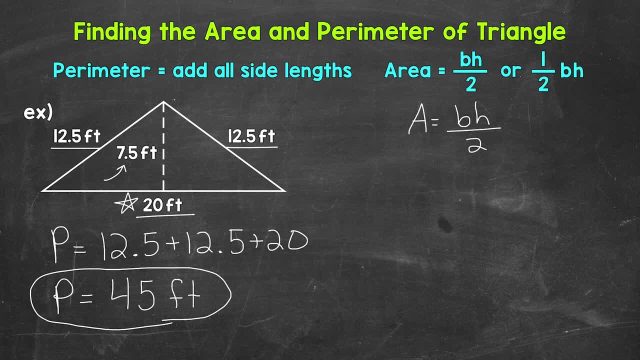 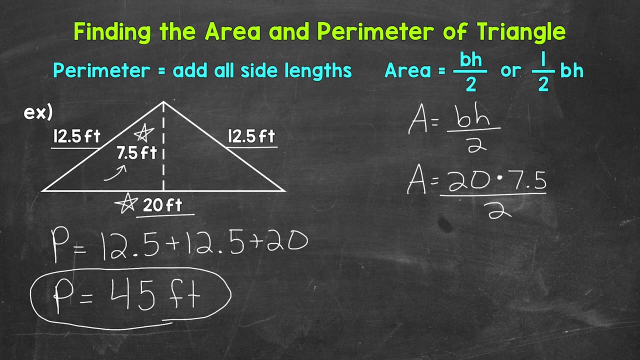 and the height. We're going to use twenty feet for the base and seven and a half feet for the height. So area equals twenty feet for the base times seven and a half feet for the corresponding height divided by two. Now we can work through this. Let's start with twenty times seven and a half. 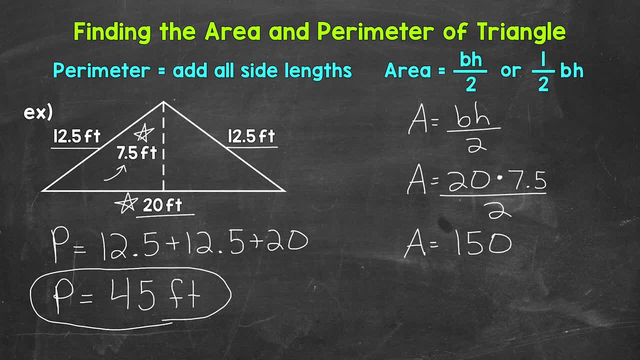